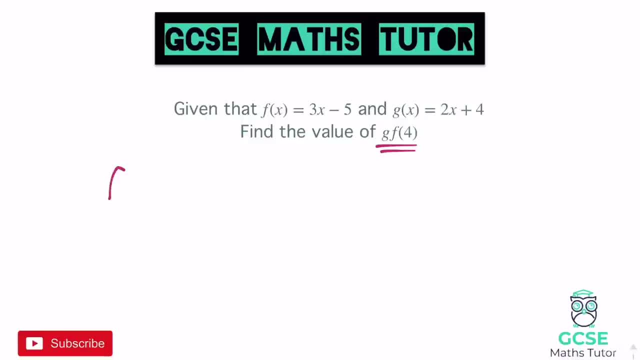 that? what is g when f is 4?? So I'm going to work out f4 to start with, which just means sub 4 into f, and if we sub 4 into f, we get 3 lots of 4, take away 5. And 3 lots of 4. 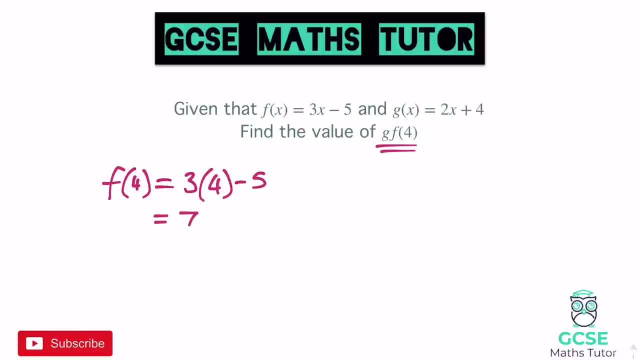 is 12, take away 5, leaves us with 7.. Okay, so when f is 4, we get the answer 7.. Now we've got 7 into g and work that out, and that gives us 2- lots of 7, 2x plus 4g is up here. 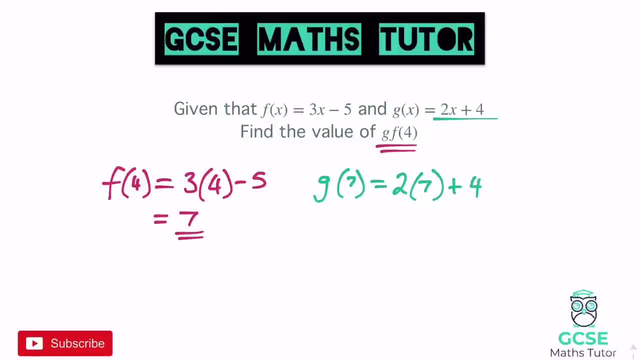 so 2, lots of 7, add 4, would give us 14 plus 4, which is 18.. There you go. So obviously, just think about the language there it was. what is g when f is 4?? Well, when f is 4, you. 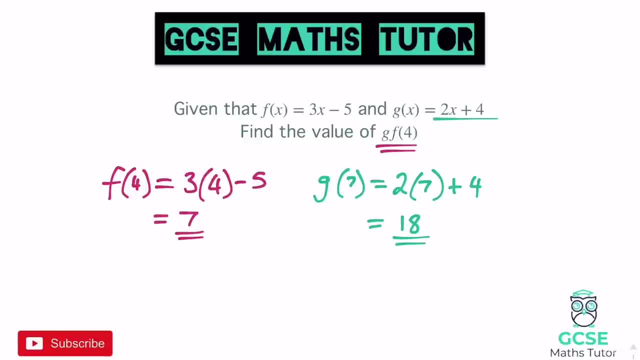 sub 4 into f and we get 3 times 4, which is 12,. take away 5, which is 7, and then, once we've got the 7 and we know what f4 is, we put that into g. 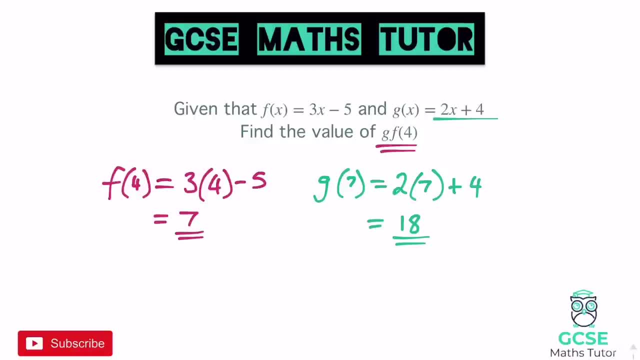 Sub that into g, which is 2, lots of 7, add the 4, so 14 add 4, give us 18.. Let's have a look at another one. Okay, so very similar question. it says: given that f of x equals: 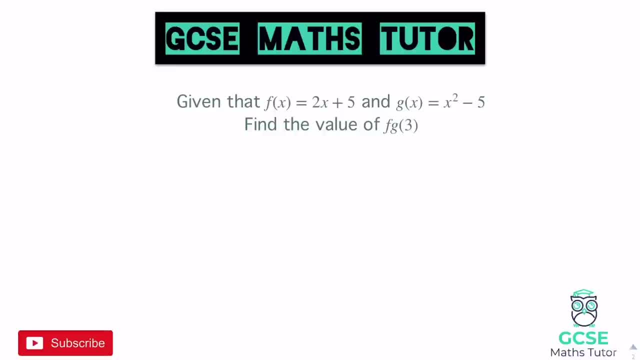 2x plus 5, and g of x equals x squared minus 5, find the value of fg3.. So letters round the other way this time, and that means what is f when g is 3, or once g is 3?? So the first. 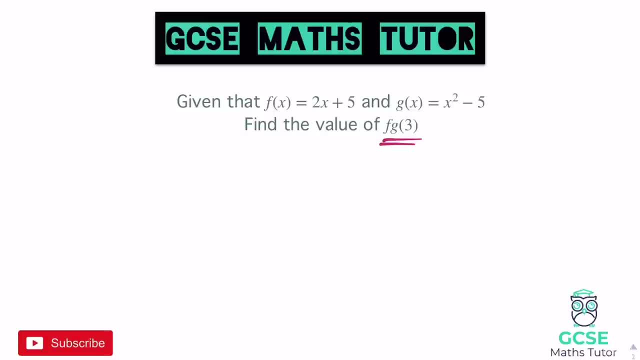 thing I'm going to have to work out is subbing 3 into g, otherwise I'm not going to be able to put the answer into f. So what is f when or once g is 3?? So sub 3 into g, we get. g3 is going to equal 3 squared x squared. this one up here, take. 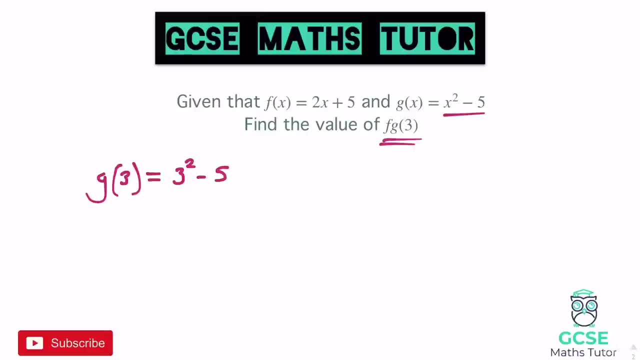 away 5.. There you go. So 3 squared is 9, take away 5, gives us the answer 4.. So 4 is what I can now put into f. so now I can work out f4, and subbing that into f. 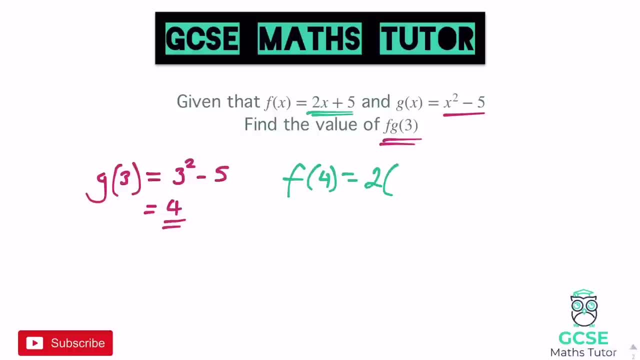 which is up here, we get 2 lots of 4, which is 8, plus 5, and 8 plus 5 equals 4.. So the answer is 13.. So you've just got to read the fg or the gf in the order and speak it as it says it. 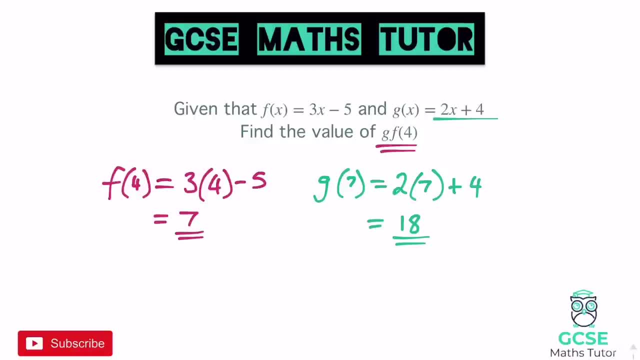 Sub that into g, which is 2, lots of 7, add the 4, so 14 add 4, give us 18.. Let's have a look at another one. Okay, so very similar question. it says: given that f of x equals: 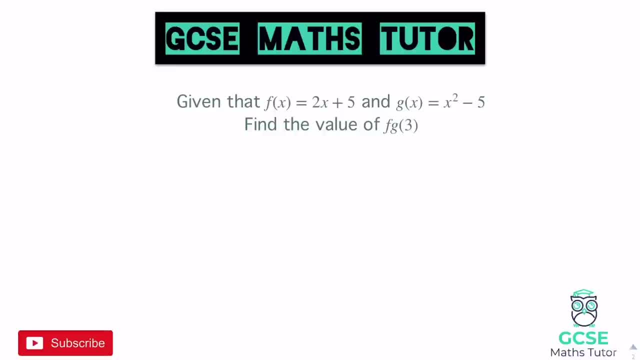 2x plus 5, and g of x equals x squared minus 5, find the value of fg3.. So letters round the other way this time, and that means what is f when g is 3, or once g is 3?? So the first. 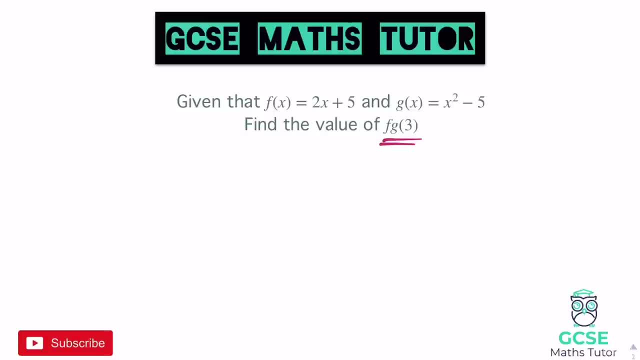 thing I'm going to have to work out is subbing 3 into g, otherwise I'm not going to be able to put the answer into f. So what is f when or once g is 3?? So sub 3 into g, we get. g3 is going to equal 3 squared x squared. this one up here, take. 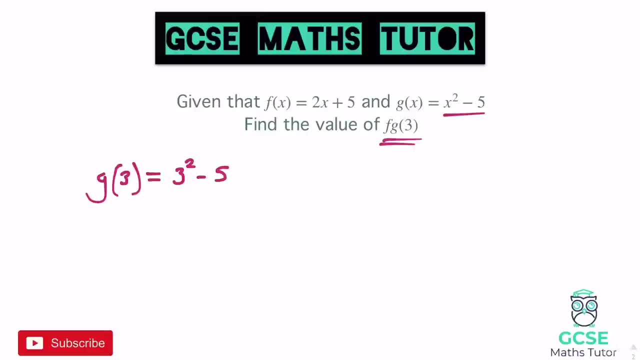 away 5.. There you go. So 3 squared is 9, take away 5, gives us the answer 4.. So 4 is what I can now put into f. so now I can work out f4, and subbing that into f. 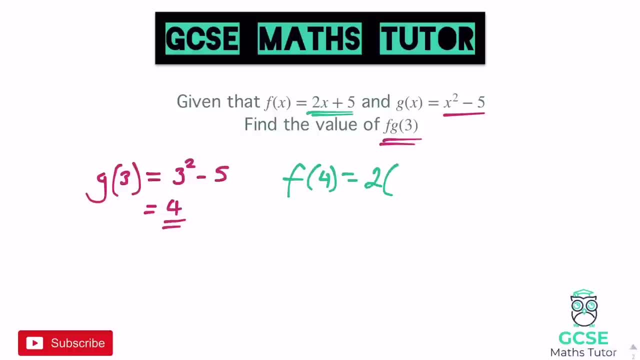 which is up here, we get 2 lots of 4, which is 8, plus 5, and 8 plus 5 equals 4.. So that's everything I've done in this example. So I'm going to take these all down now and I'm going to put them in this table and I'm 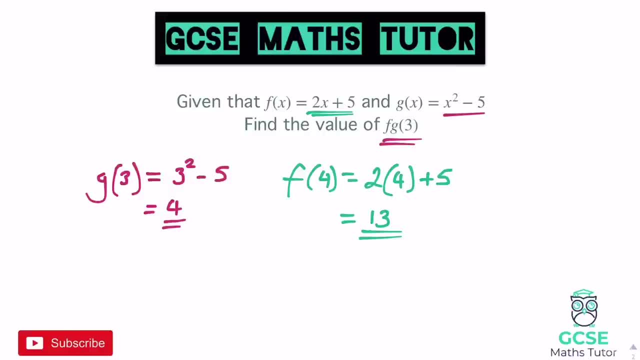 going to look at the same table as I did for my whole video. So here's a table, and here's a table with 4 legs, and there are 5 legs. and here's a table that has 6 legs, and here's a table that has 8 legs, and here's a table that has 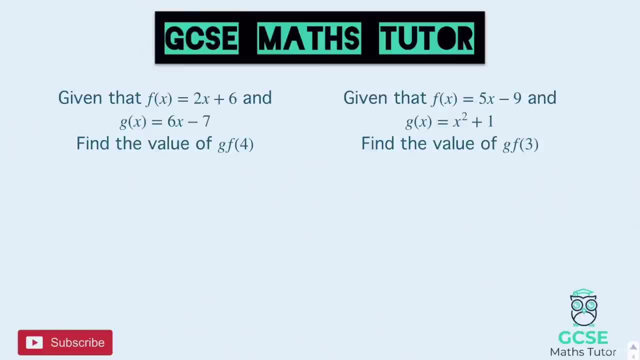 3 legs. So if I have my 2 legs and I start up on my left like this, and I've got 3 legs, I've got 8 legs, I've got 5 legs, I've got 7 legs. 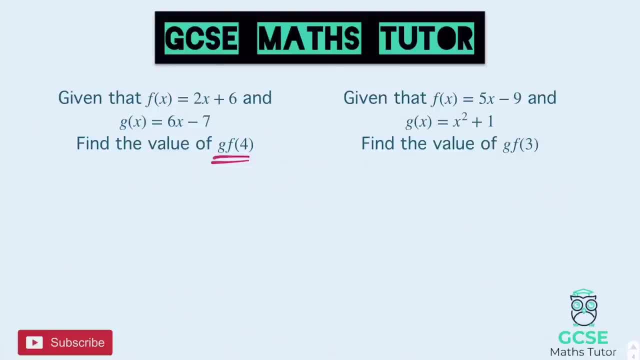 So that's the first thing I've done. I've got 4 legs, so I'm going to work that out. What is g when f is 4?? So let's work out f4 to start with. So, subbing 4 into f, we get 2 lots of 4 plus 6, 2 lots of 4 is 8, plus 6 is 14, there we. 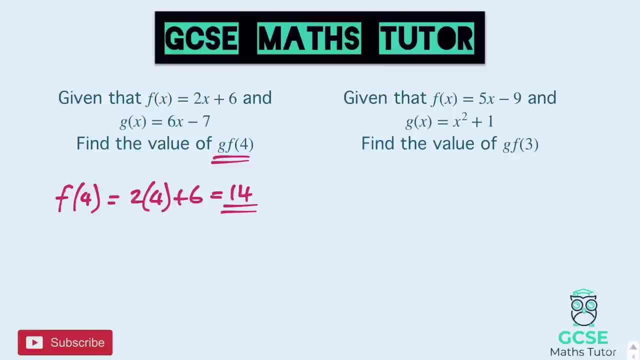 go. So we get 14. when we put 4 into f, That's the number we're going to put into g. so g14, not the nicest one here, because we have 6, lots of 14, then we have to take away 7, there we go. 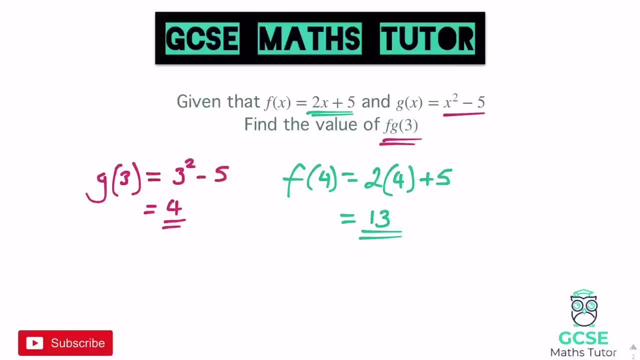 So f of g three means the function of g, sorry, the function of f when g is 3.. So let's have a look and some questions for you to have a go at. Okay, so here are two questions, So have a go at these two. pause the video there. we'll give you the answer in a sec. 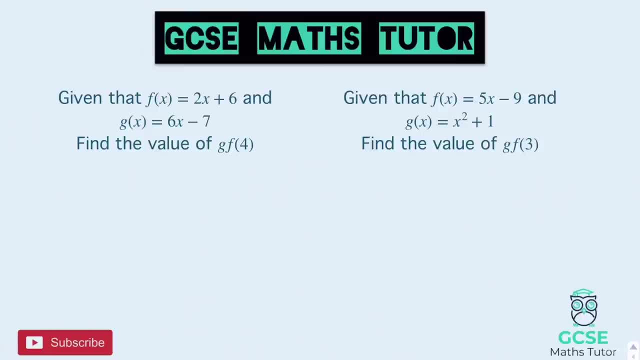 Okay, so this first one on the left. It says find gf4.. So what is g? It's a symbol when f is 4.. So let's work out f4 to start with. So, subbing 4 into f, we get 2, lots of 4. 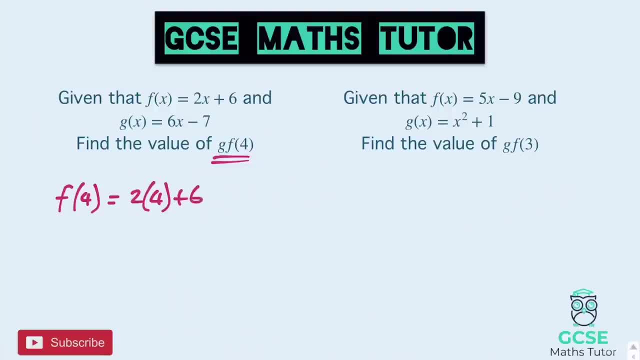 plus 6.. 2 lots of 4 is 8 plus 6 is 14.. There we go, So we get 14. when we put 4 into f, That's the number we're going to put into g, So g14.. Not the nicest one here, because we have 6. 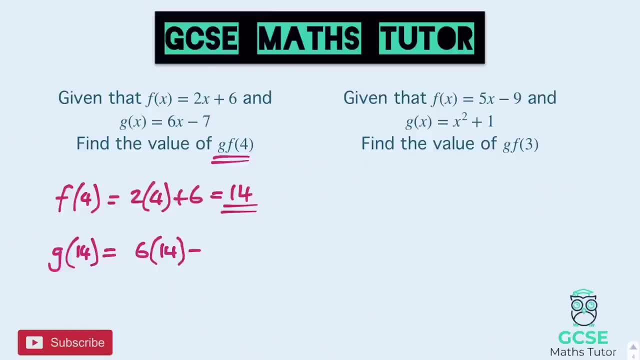 lots of 14.. Then we have to take away 7.. There we go. Obviously, we have got quite a large number there, bigger than before. So just go back, double check, make sure you're happy with that. That said, what is g when f is 4?? We've put 4 into f. 2 lots of 4 is 8 plus 6 is 14.. Okay, absolutely fine with. 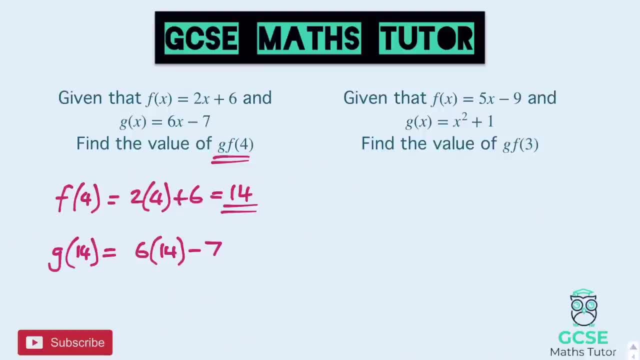 that. So 14 is what's going into g. So we need to work this out: 6 times 14, or 6 times 10, is 60.. 6 times 4 is 24.. So that's 84.. So 84 take away 7.. 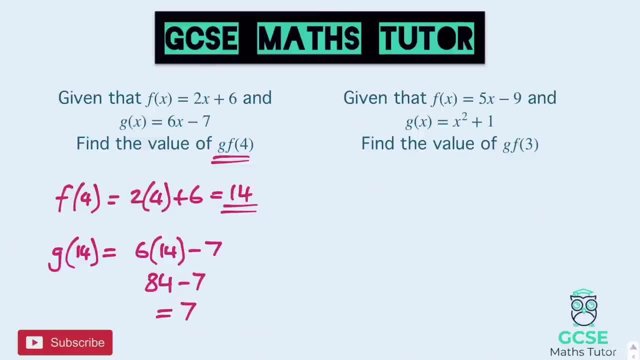 And 84 take away 7.. 7 leaves us with 77.. There we go, and 77 is our final answer. On to the next one, It wants us to find gf3.. So we're going in. We want to know what is g when f is 3.. So the same way around again. 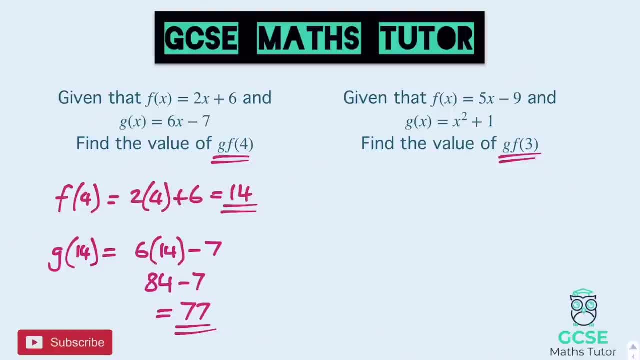 actually. So you've just got to watch out, obviously, if I've done one of each here. But let's have a look. We need to find g when f is 3.. So let's put 3 into f, So f3, and that's going to give us 15.. 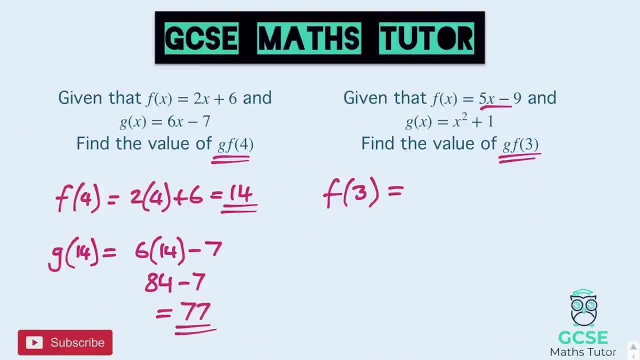 5 lots of 3.. This f up here- 5 lots of 3- is 15.. Let's write it down: Take away 9.. So 15 take away 9 equals 6.. There we go. So it's 6 that we are going to be putting into g, So into g with 6.. And that's going. 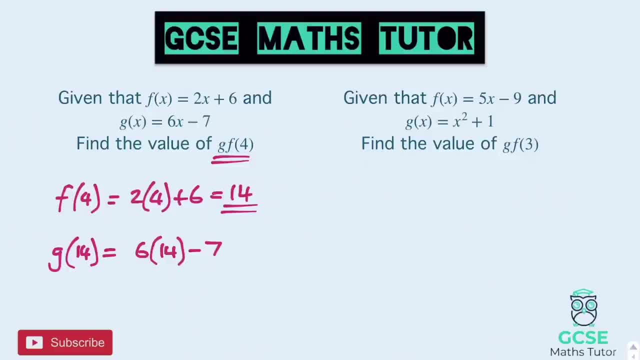 Obviously we have got quite a large number there, bigger than before. so just go back double check, make sure you're happy with that. that said, what is g when f is 4?? We've put 4 into f. 2. lots of 4 is 8, plus 6 is 14,. okay, absolutely fine with that. 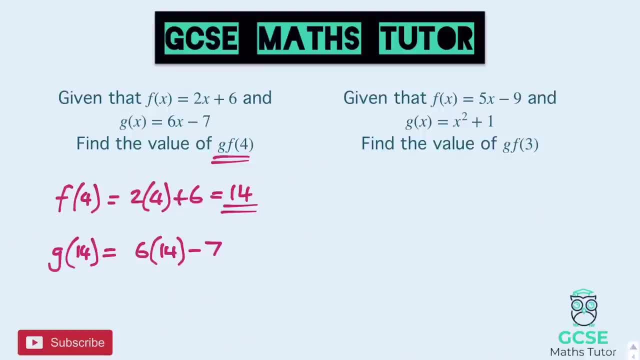 so 14 is what's going into g. So we need to work this out. 6 times 14, or 6 times 10, is 60,, 6 times 4 is 24, so that's 84, so 84 take away 7, and 84 take away 7 leaves us with 77,. there we go, and 77 is. 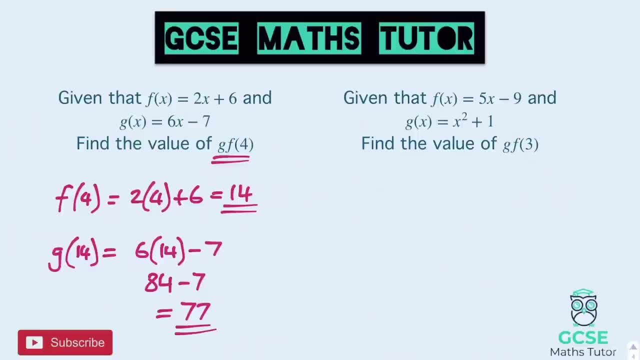 our final answer On to the next one. it wants us to find gf3, so we're going in. we want to know what is g when f is 3, so the same way around again, actually. so you've just got to watch out. 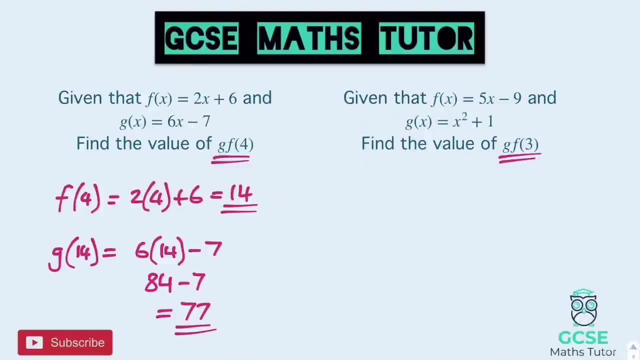 obviously if I've done one of each here. but let's have a look. We need to find g when f is 3, so let's put 3 into f, so f3, and that's going to give us 15,, 5 lots of 3, using this f up here, 5 lots of 3 is 15, let's write it down, take: 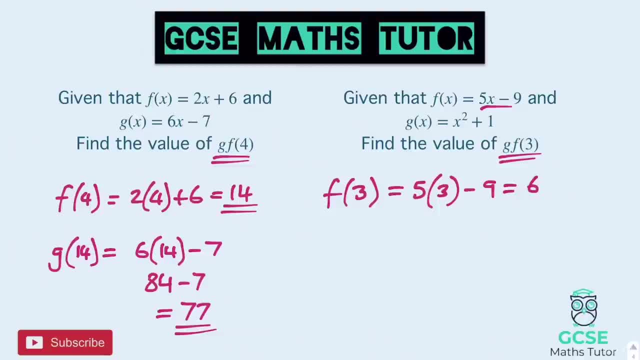 away 9.. So 15 take away 9 equals 6, there we go. so it's 6 that we are going to be putting into g, so into g with 6, and that's going to be x squared plus 1, the second one. so we've. 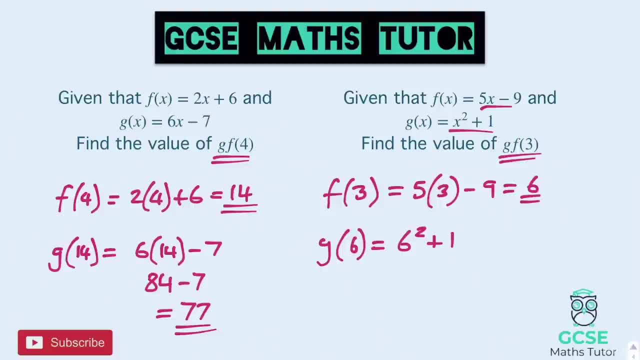 got 6 squared plus 1,. 6 squared is 36, so we have 36 plus 1, and our answer there is 37,. okay, So obviously just being careful what it says. obviously, if that had have said fg3, it would. 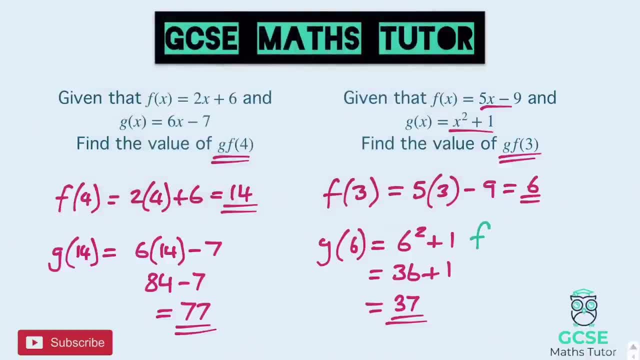 have done that in a different way, okay. So if it had have said fg3,, we'd have first put 3 into g, and g3 would have given us 3 squared plus 1,. 9 plus 1 equals 10, and then we'd have put 10 into f. if it was the other. 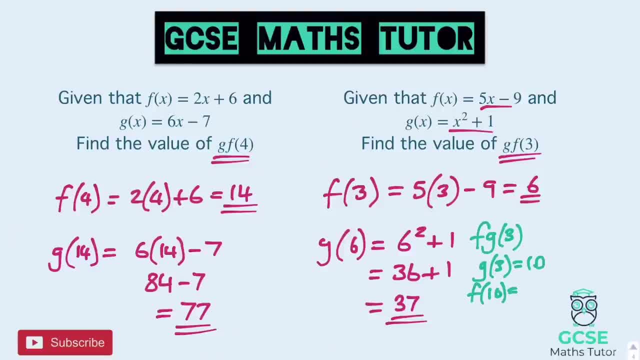 way around. so we'd have done f10, and that would have been 5 times 10 is 50, take away 9, 50, take away 9 is 41, so you've got the answer: 41 doing it the other way around, okay. 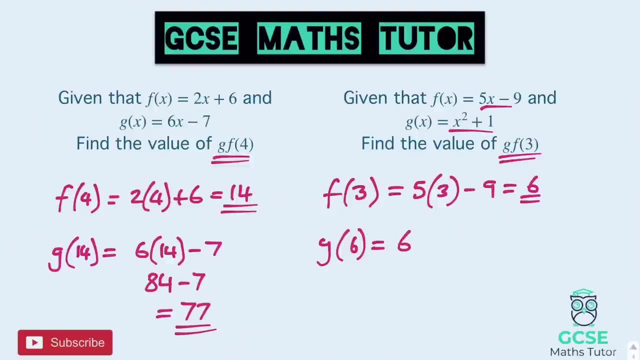 to be x squared plus 1.. The second one. So we've got 6 squared plus 1.. 6 squared is 36.. So we have 36 plus 1. And our answer there is 30. 7. Okay, So obviously just being careful what it says. Obviously, if that had have said fg3, we'd have 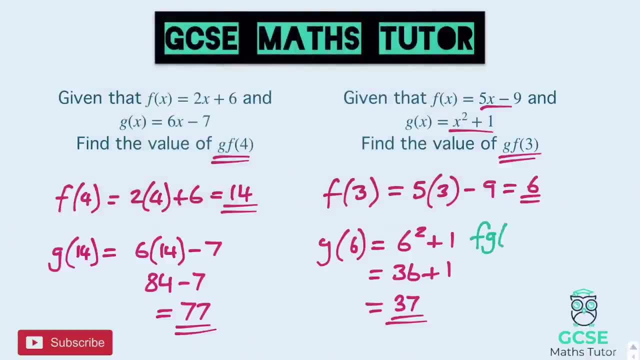 done that in a different way. Okay, So if it had have said fg3, we'd have first put 3 into g, And g3 would have given us 3 squared plus 1.. 9 plus 1 equals 10.. And then we'd have put 10 into f. if it. 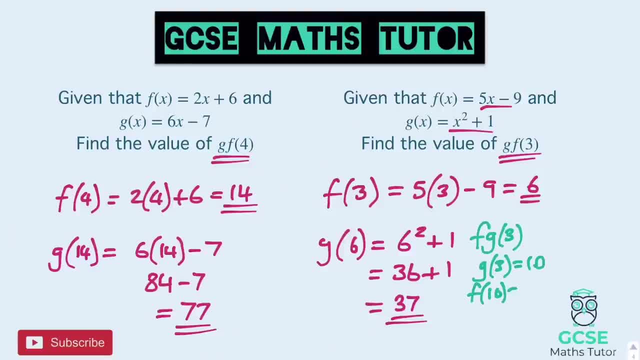 was the other way around, So we'd have done f10. And that would have been 5 times 10 is 50. Take away 9.. 50, take away 9 is 41. We've got the answer: 41 doing it the other way around. Okay, So just be very careful what the 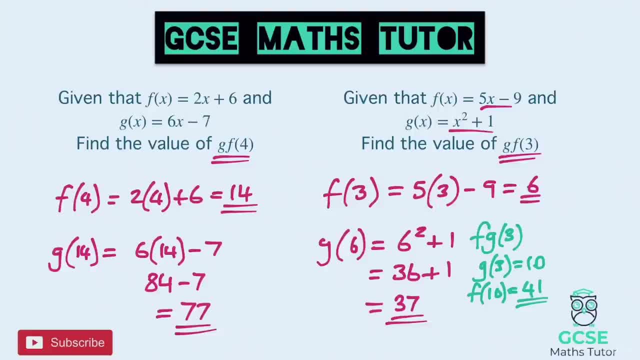 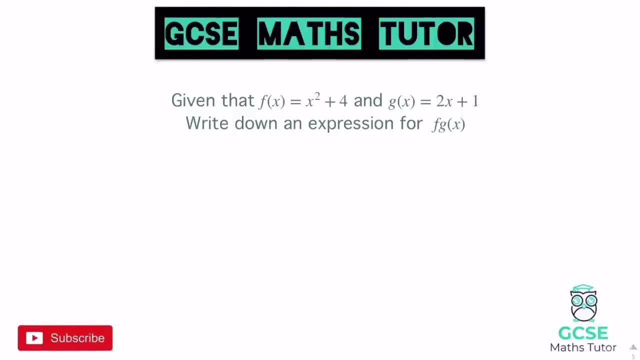 language says The way the letters are organised there. Let's have a look at what happens when there's not any numbers in them. Okay, So this question here says: given f of x is x squared plus 4 and g of x is 2x plus 1.. Write down an expression for fgx. Okay, So we're not putting a number in. 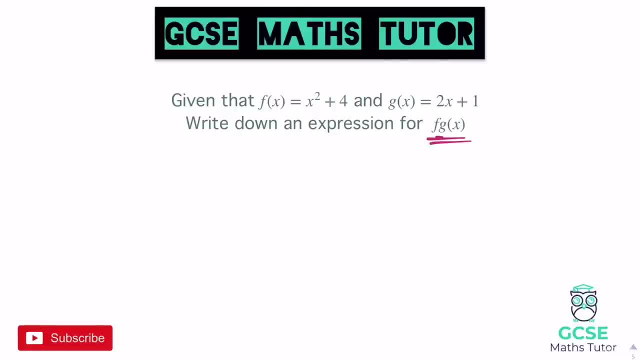 this time It says: write down an expression for fgx. So that means what is the function of f when you put g into it? Okay, So not any numbers or anything. Just what is f when you put somewhere? sub the function g in. So if I want to sub the function g into f, there's a nice little trick for. 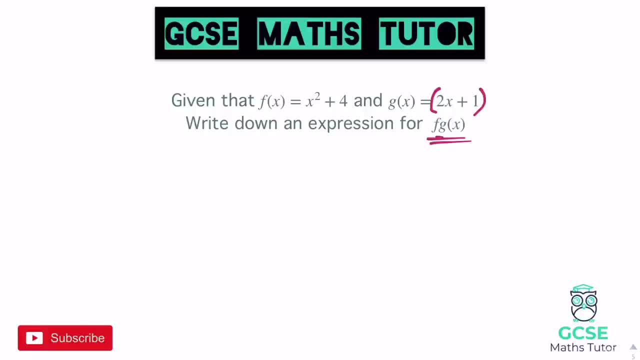 it. I'm just going to put a bracket around the whole function. I'm going to put it in the place of the x in f. So if I actually do that, Let's actually put that in there. If I just put the bracket in, So 2x plus 1. It's x squared, So that bracket is squared plus 4.. Now that is actually an. 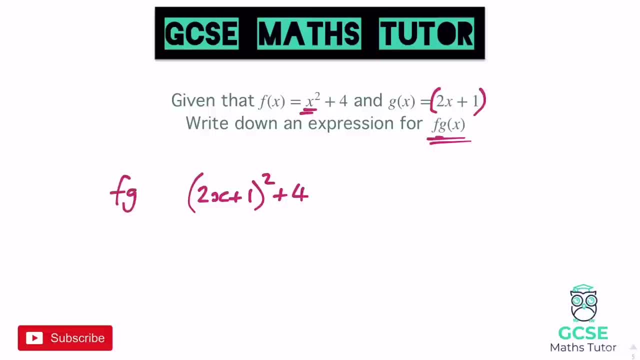 expression there for fgx. That's absolutely fine fgx. But normally we would go and expand this and tidy it all up. So obviously, if I do want to do that now to tidy it all up, we've got a double bracket to expand there. So we have 2x plus 1.. 2x plus 1.. And at the end of all that we need to add: 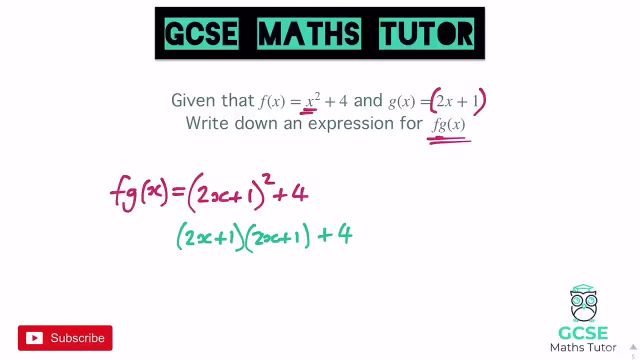 4 to the end. So expand that as a double bracket. 2x times 2x is 4x squared, That's that one, And we've got 2x times 1 and 1 times 2x And that's going to give us a 2x and a 2x, which makes 4x. 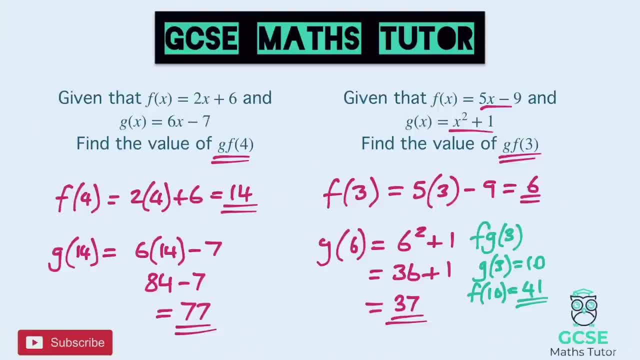 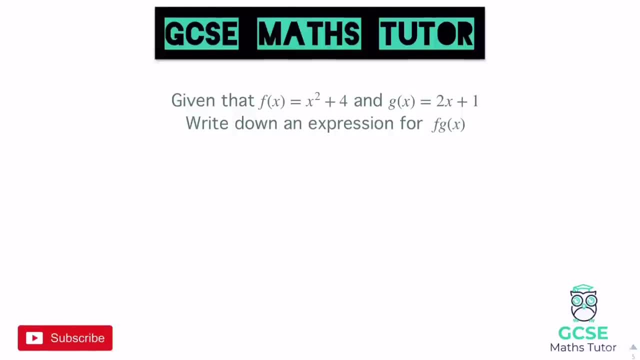 So you've just got to be very careful what the language says, the way the letters are, the way the numbers are organised there. Let's have a look at what happens when there's not any numbers in them. Okay, so this question here says: given f of x, is x squared plus 4, and g of x is 2x. 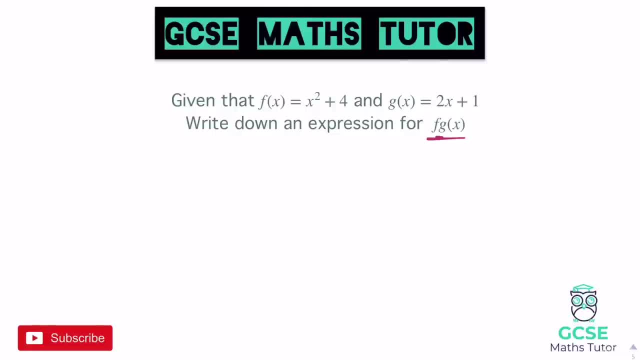 plus 1, write down an expression for fgx. okay, So we're not putting a number in this time. it says write down an expression for fgx. so that means what is the function of f when you put g into it? okay, 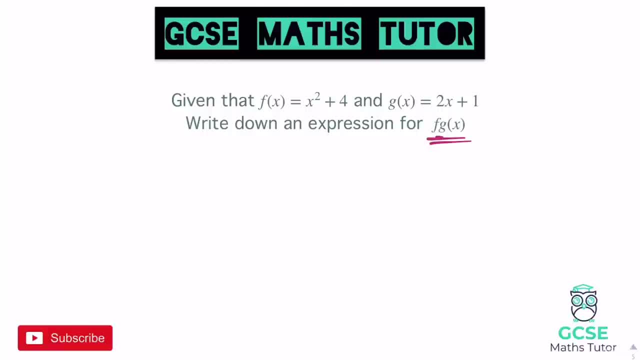 So not any numbers or anything, just what is f when you put, when you sub the function g in. So if I want to sub the function g into f, there's a nice little trick for everyone. okay, I'm just going to put a bracket around the whole function. I'm going to put it in the 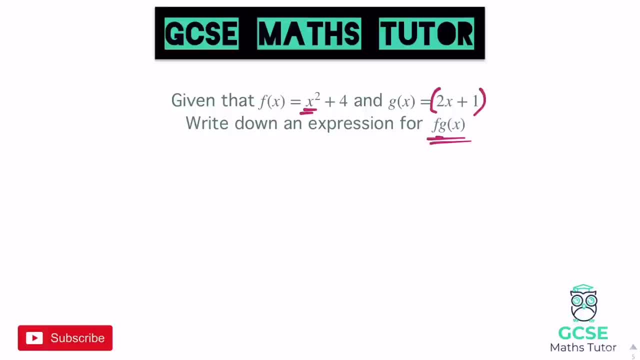 place of the x in f. So if I actually do that, let's actually put that in there. if I just put the bracket in, so 2x plus 1, it's x squared, so that bracket is squared plus 4, now that is actually an. 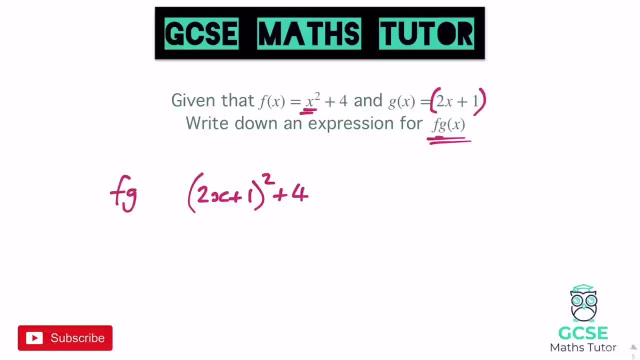 expression there for fgx. that's absolutely fine fgx. but normally we would go and expand this and tidy it all up. so obviously, if I do want to do that now to tidy it all up, we've got a double bracket to expand there. so we have 2x plus 1, 2x plus 1, and at the 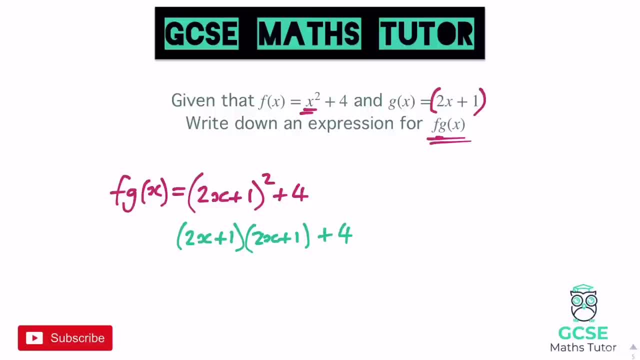 end of all that, we need to add 4 to the end, So expand that as a double bracket. 2x times 2x is 4x squared, that's that one and we've got 2x times 1 and 1 times 2x and that's going to give us a 2x and a 2x, which makes 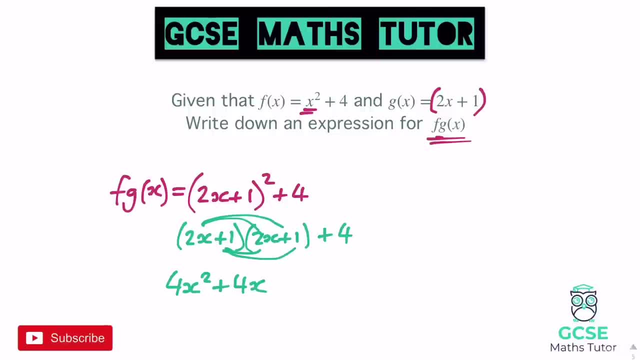 4x and the final multiplication there: 1 times 1 gives us 1, and we're going to add 4 at the end. So tidying this all up, getting that nice expression there: Okay, We've got 4x squared plus 4x. and then 1 plus 4 gives us plus 5 at the end, so 4x squared. 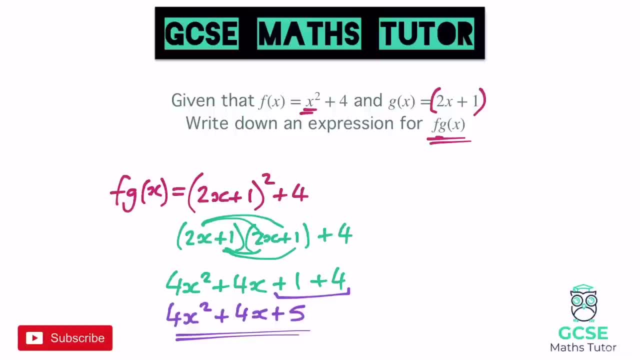 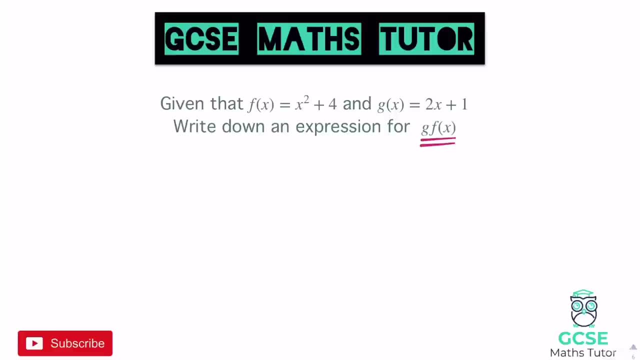 plus 4x plus 5.. Let's have a look at another one where it's the other way around. so same functions here, but we have a look at gfx. Okay, so we've got gfx this time. let's see how it's different if we do it like this. 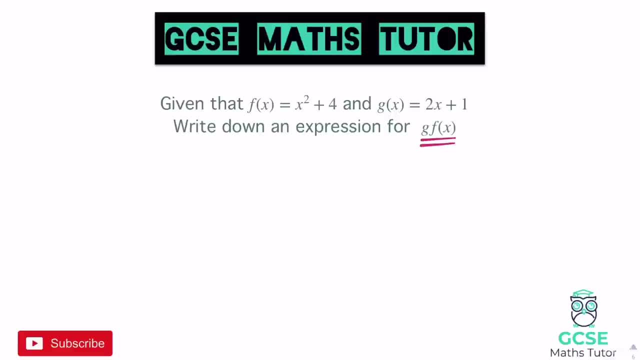 So this means what's g when we put f in? So I'm going to put my bracket around the f function, I'm going to sub that into g. So we've got 2, lots of g, Lots of that bracket, 2 lots of x squared plus 4, and then at the end we've got plus. 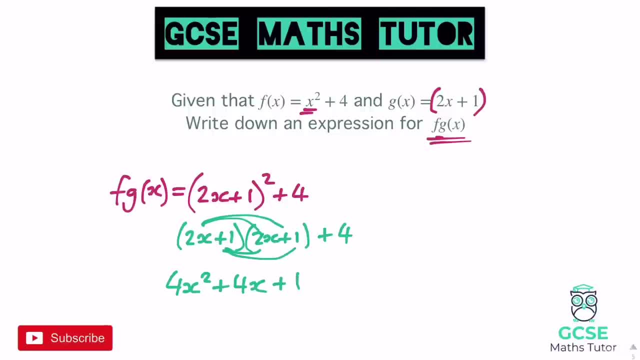 And the final multiplication there: 1 times 1 gives us 1. And we're going to add 4 at the end. So tidying this all up, Getting that nice expression there, We've got 4x squared plus 4x. And then 1 plus 4 gives us plus 5 at the end. So 4x squared plus. 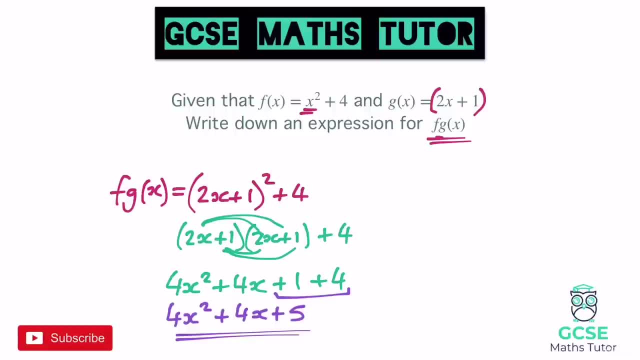 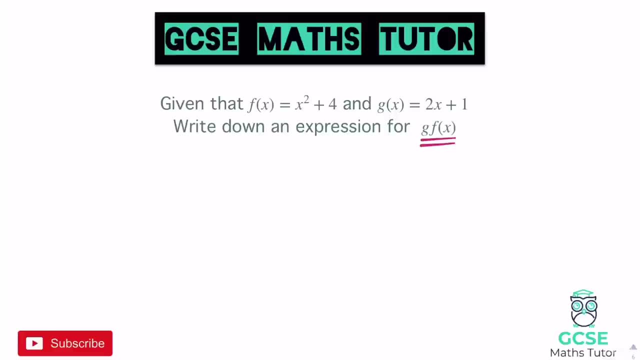 4x plus 5.. Let's have a look at another one where it's the other way around. So same functions here, but we have a look at gfx. Okay, so we've got gfx this time. Let's see how it's different if we do it like this. So this means what's g when we put f in? So I'm going. 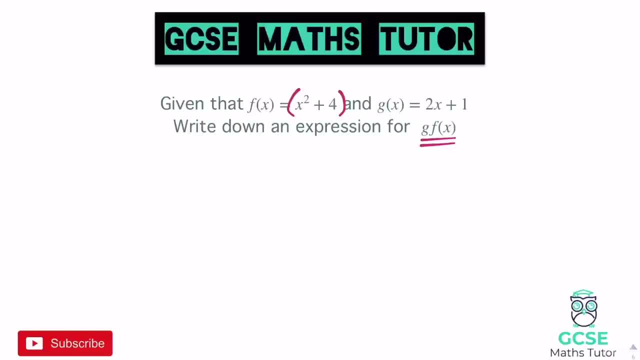 to get around the f function, I'm going to sub that into g. So we've got 2, lots of that bracket, 2, lots of x squared plus 4.. And then at the end we've got plus 1.. So I just need to tidy this. 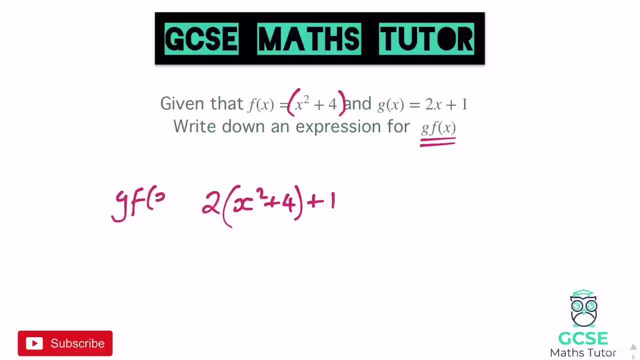 all up now, And that's going to give me my expression for gfx. There we go. So let's just times this bracket out: 2 lots of x squared is 2x squared. 2 lots of 4 is 8.. I'm not forgetting. 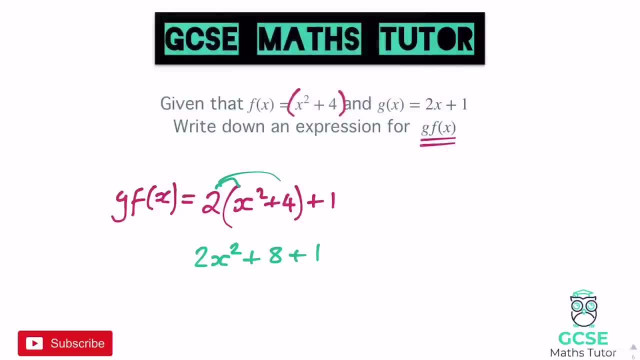 to add the 1 at the end, And then we just need to tidy all this up. So we're going to add the 1 at the end. Add these two bits together and we get 2x squared plus 9.. And that's our expression there for gfx. 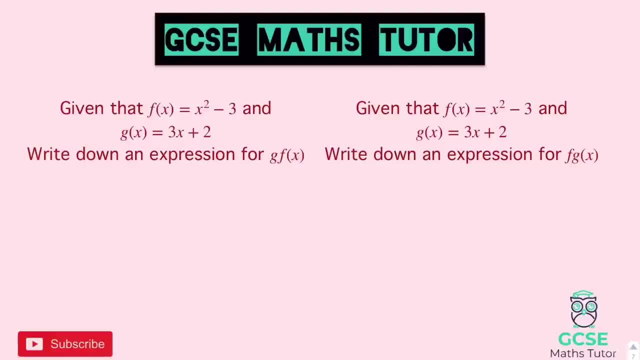 Right, okay, here's something to have a go at. Okay, so two questions. Have a go at both of these and we'll go over the answers in a sec. Okay, so the first one says gfx. So it's important in the order you do these, because these are the same two functions in both of them, But it's important we. 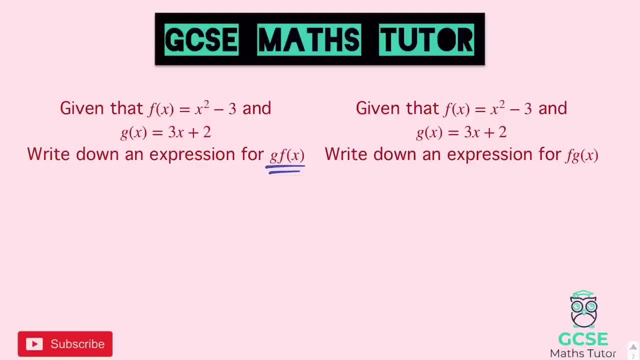 get it the right way around. So this means: what is g when we put f in? So for the first one we need to get f when we put g in, So we have 3, lots of x squared minus 3.. And then plus 2 at the end. 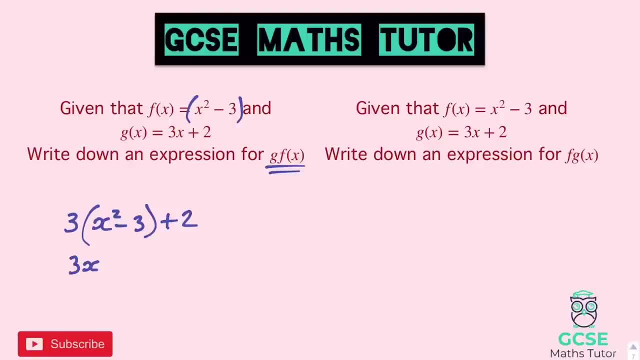 And expanding all that out, we get 3x squared minus 9 plus 2.. And tidying that up for the last step: 3x squared minus 9, add 2 is minus 7.. So 3x squared minus 7.. Onto the other one, we have fgx. 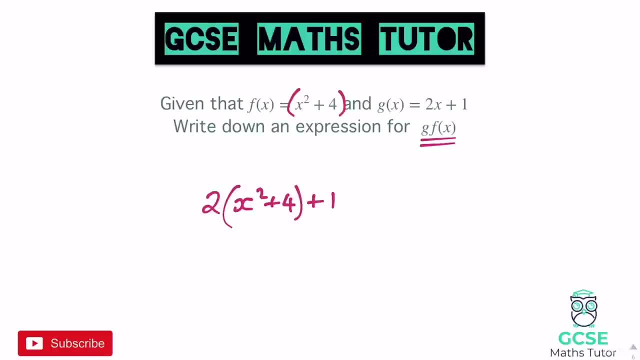 1. So I just need to tidy this all up now, and that's going to give me my expression for gfx. There we go. So let's just times this bracket out: 2 lots of x squared is 2x squared. 2 lots of 4 is. 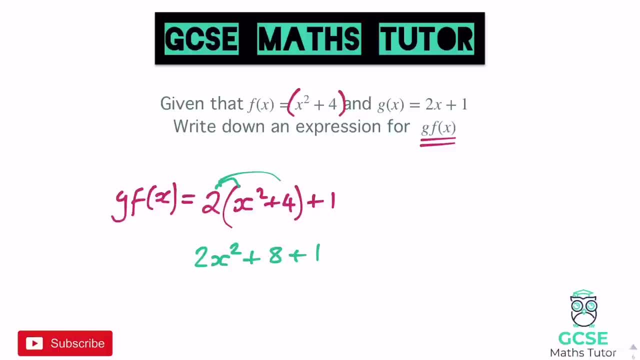 8, and not forgetting to add the 1 at the end, and then we just need to tidy all this up. So we're going to add these two bits together and we get 2x squared plus 4x squared 9.. 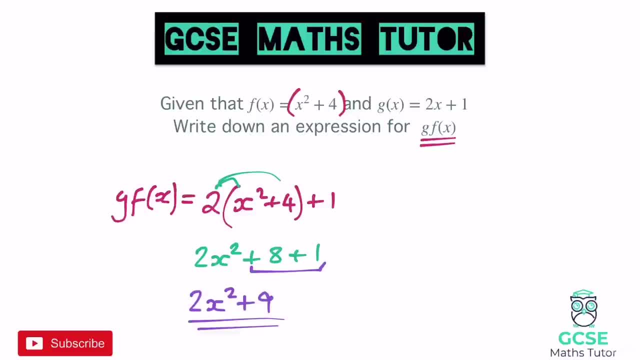 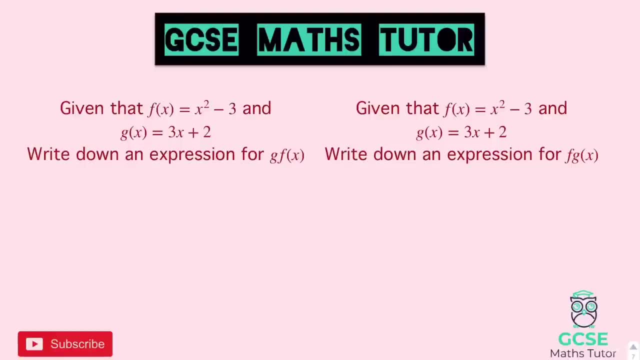 And that's our expression there for gfx, Right, okay, here's something for you to have a go at. Okay, so two questions. have a go at both of these and we'll go over the answers in a sec. Okay, so the first one says gfx. so it's important in the order you do these, because these are 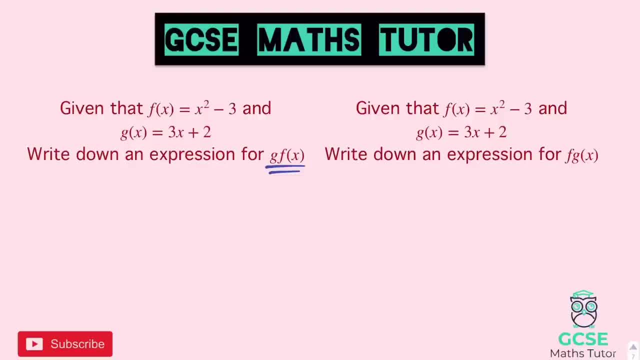 the same two functions in both of them, but it's important we get it the right way round. So this means what is g when we put f in? So for the first one we need to put our brackets around the f function and sub it into g. 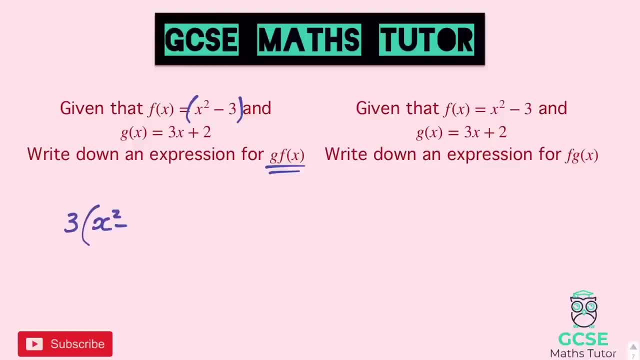 So we have 3 lots of x squared minus 3.. So we've got 3 lots of x squared minus 3.. So we've got 3 lots of x squared minus 3.. And then plus 2 at the end And expanding all that out, we get 3x squared minus 9 plus 2.. 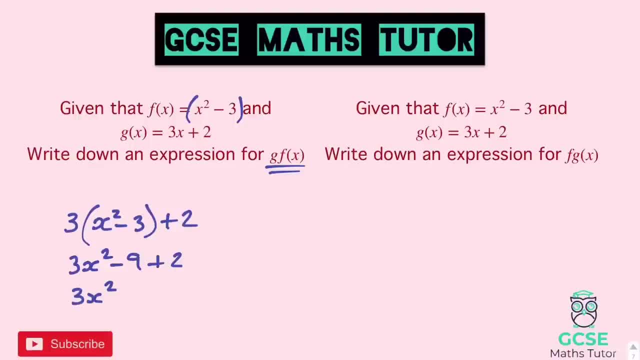 And tidying that up for the last step: 3x squared minus 9, add 2 is minus 7, so 3x squared minus 7.. Onto the other one. we have fgx. so what is f when we put g in? 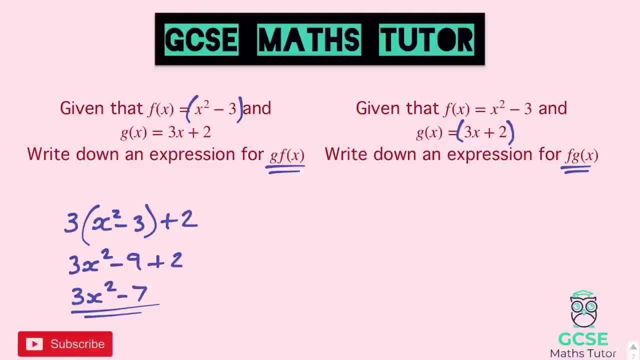 So this time brackets around the g and subbing that in, So it's x squared. so we've got 3x plus 2 squared, Okay, And then minus 3 at the end And expanding that as a double bracket, there we're going to get 9x squared plus 6x plus. 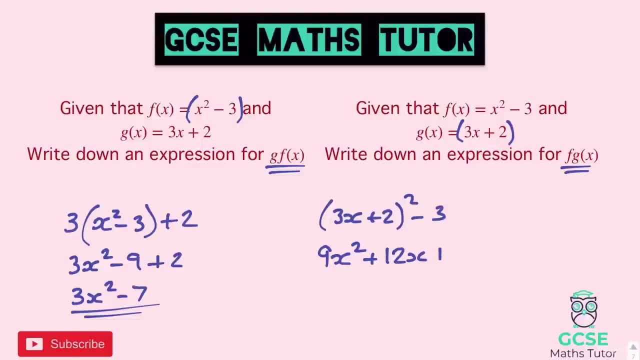 6x, which gives us plus 12x. 2 times 2 will give us 4, and then minus 3 at the end. And again, just tidy that up, We can write the full double bracket out, but we get 9x squared plus 12x plus 4 minus. 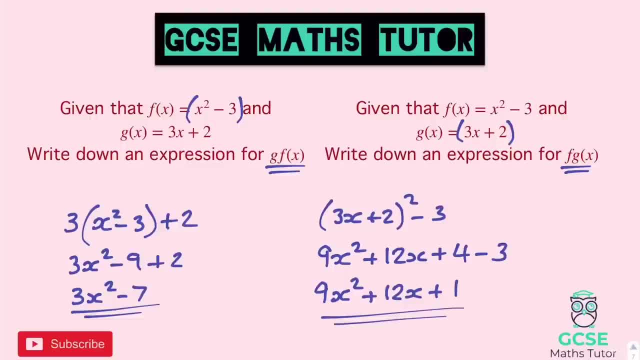 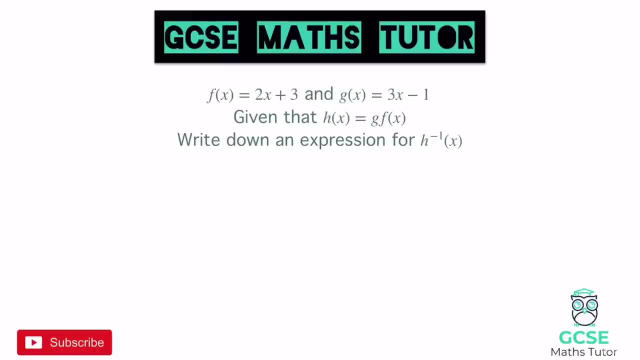 3 is plus 1.. And there's our expression there for fgx. Now, before we finish, I've got one more for you to have a look at. So we've got fgx, Okay. And the last question here: f of x equals 2x plus 3, and g of x equals 3x minus 1.. 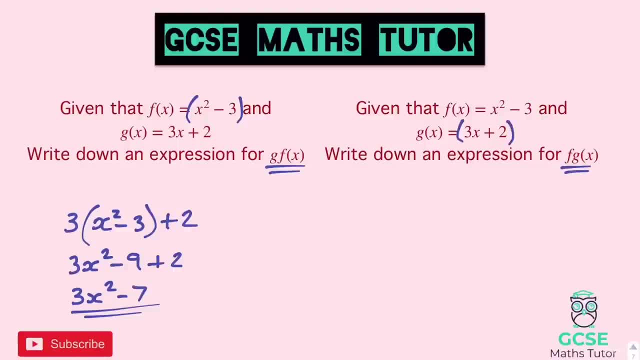 So what is f when we put g in? So this time brackets around the g And subbing that in So it's x squared. so we've got 3x plus 2 squared and then minus 3 at the end and expanding that as a double bracket. 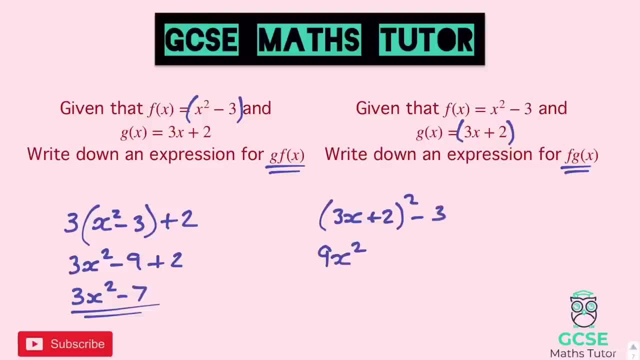 there we're going to get 9x squared plus 6x. plus 6x, which gives us plus 12x. 2 times 2 will give us 4 and then minus 3. at the end and again, just tidy that up- you can write the full double bracket. 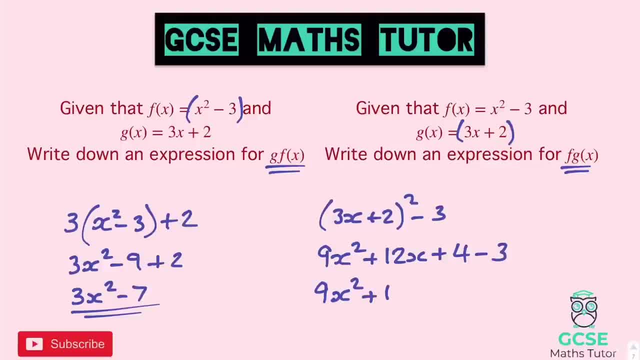 out, but we get 9x squared plus 12x plus 4. minus 3 is plus 1, and there's our expression there for fgx. Now, before we finish, I've got one more for you to have a look at. Okay, and the last question. 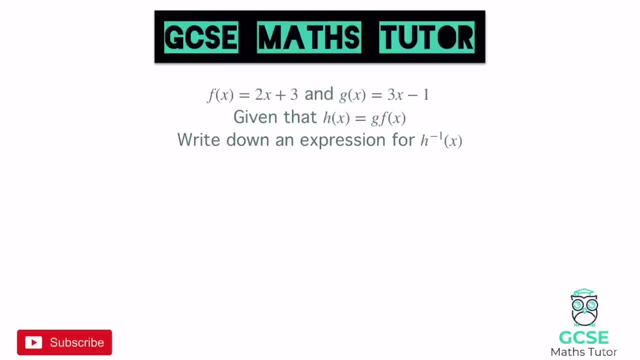 here, f of x equals 2x plus 3 and g of x equals 3x minus 1. given that h of x, which is just another function that's not given to us, is the same as or equal to gfx, write down the expression for the: 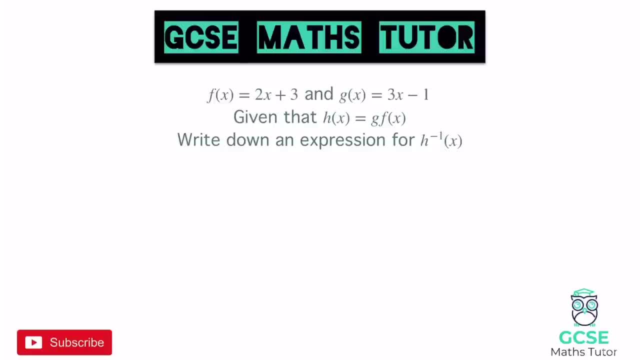 inverse function of h. so obviously there is a bit of inverse functions in this as well. so you will have to have a good knowledge of inverse functions here, which I'll link in the description on the video on that. but have a go at this question. see what you get. it doesn't matter if you get. 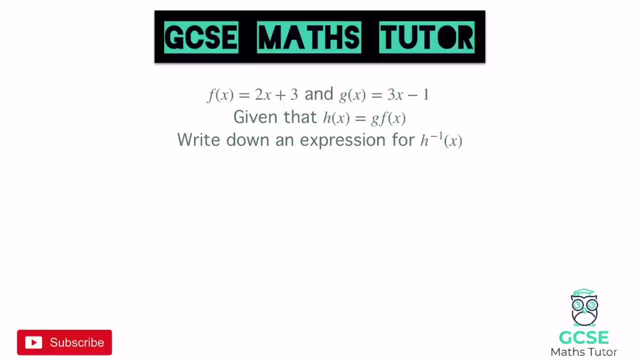 it wrong. I'm going to go over the answers in a sec, but pause the video there. have a go and we'll go over the answer. Okay, so it says: given that h of x equals gfx. so first things first, let's find out what gfx is, and that's the function of g when we put f in, so brackets around the f and let's sub. 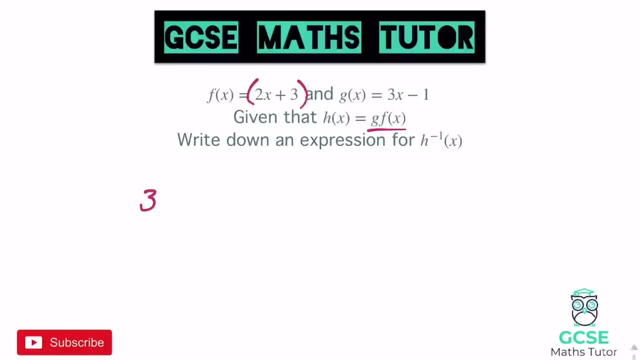 that in, so we get three lots of. obviously just putting it into the x here, we get three lots of 2x plus 3. take away 1 and if we expand that out we get 6x plus 9, but then take away 1. let's write that in two steps: plus 9 minus 1, which is 6x plus. 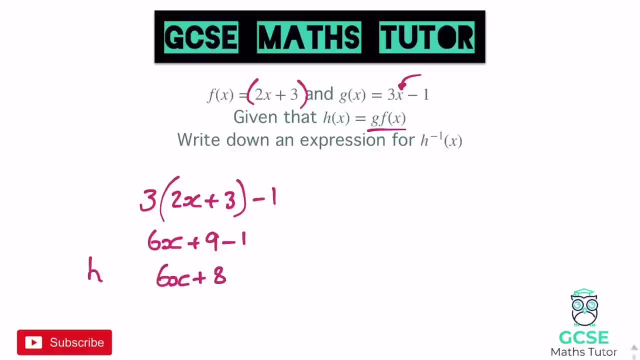 8, and that is the function of h. so h of x equals 6x plus 8. now it wants us to find the inverse function of h. okay, so let's just work that out and to find the inverse function, we're going to write it as y equals, so y equals 6x plus 8, and let's make x the subject, so y minus 8. 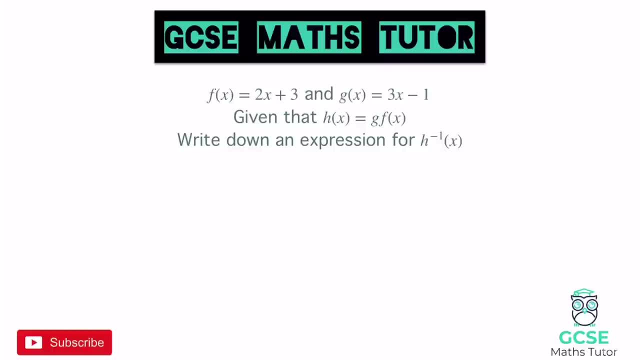 Given that h of x, which is just another function that's not given to us, is the same as or equal to g of x, write down the expression for the inverse function of h. So obviously there is a bit of inverse functions in this as well. 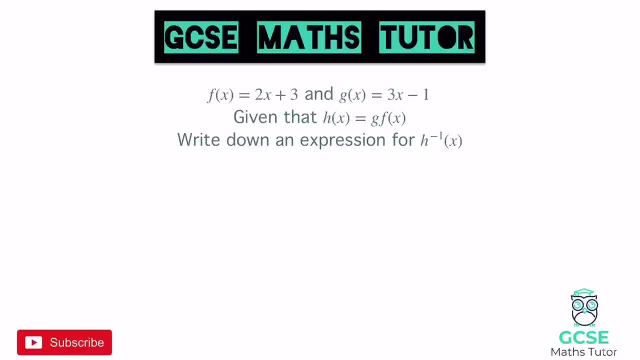 So you will have to have a good knowledge of inverse functions here, which I will link in the description on the video on that. But have a go at this question. See what you get. It doesn't matter if you get it wrong. I'm going to go over the answers in a sec. 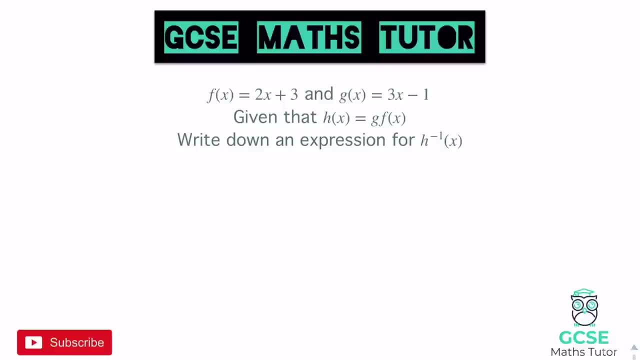 But pause the video there. Have a go and we'll go over the answers. Okay, so it says, given that h of x equals g of x. so first things first, let's find out what g of x is, And that's the function of g when we put f in. 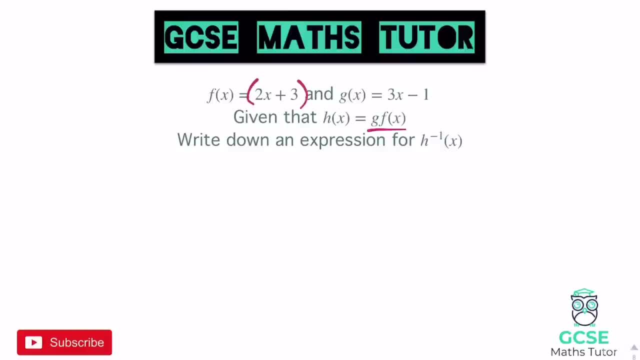 So brackets around the f and let's sub that in, So we get 3 lots of obviously. just putting it into the x here we get 3, lots of 2x plus 3, take away 1. And if we expand that out we get 6x plus 9.. 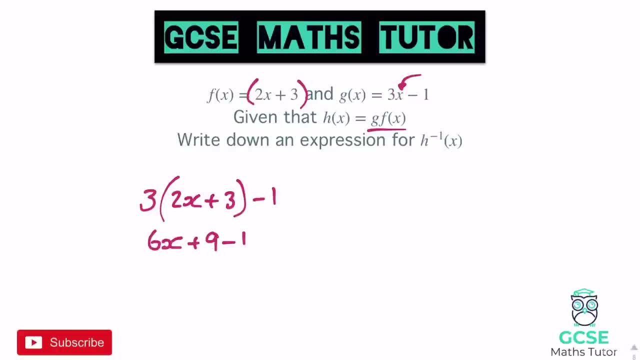 But then take away 1, let's write it out in two steps: plus 9 minus 1, which is 6x plus 8.. And that is the function of h. So h of x equals 6x plus 8.. 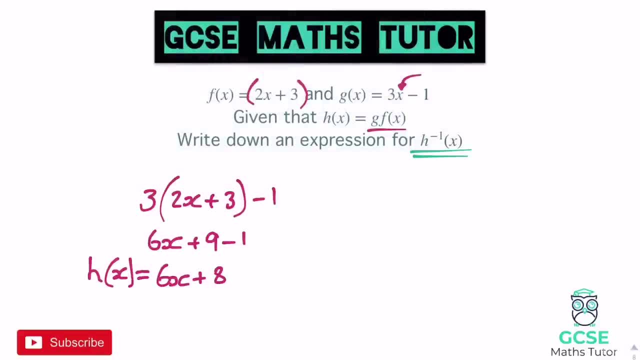 Now it wants us to find the inverse function of h. Okay, so let's just work that out. And to find the inverse function, we're going to write it as y equals, so y equals 6x plus 8.. And let's make x the subject. 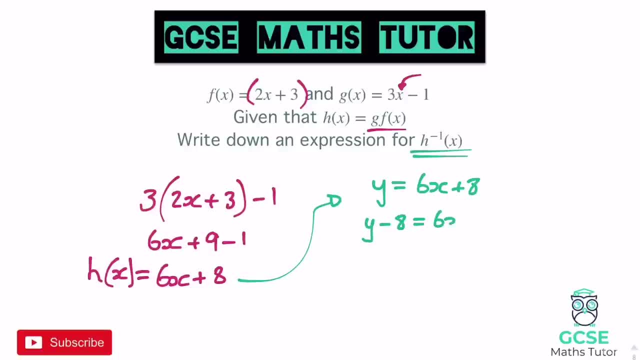 So y minus 8 equals 6x, And then divide that by 2. And then divide by 6. So y minus 8 over 6 equals x. And then let's swap around the x and y's. So x minus 8 divided by 6 equals this inverse function of h. 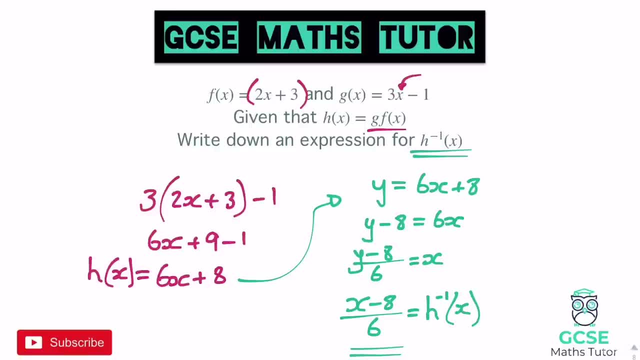 There we go. So something that looks a little bit more complicated there, but that is our inverse function: x minus 8 over 6.. Okay, so that is the end of composite functions. Again, if you found that useful, if you found it helpful, please like, please comment, please. 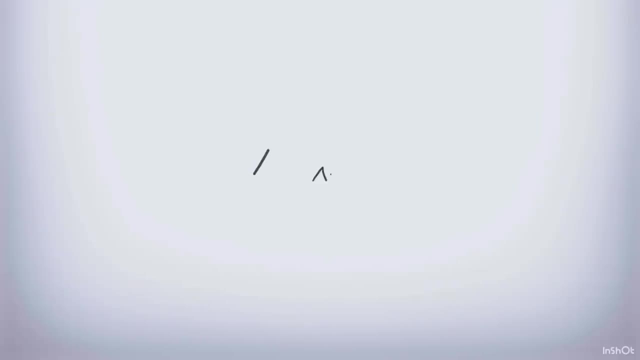 subscribe and I'll see you on the next video. Bye for now, Bye, Bye, Bye, Bye, Bye, Bye.